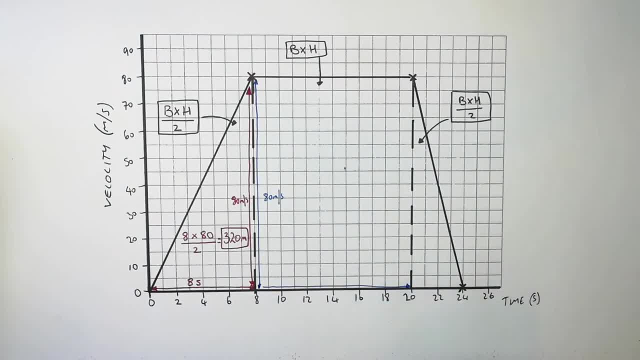 meters per second. So to work out the base it's going to be, it's going to be 20 seconds minus 8 seconds. 20 seconds minus 8 seconds, That gives you a time of 12 seconds. So the base is 12 seconds. So that means to work out the distance, the 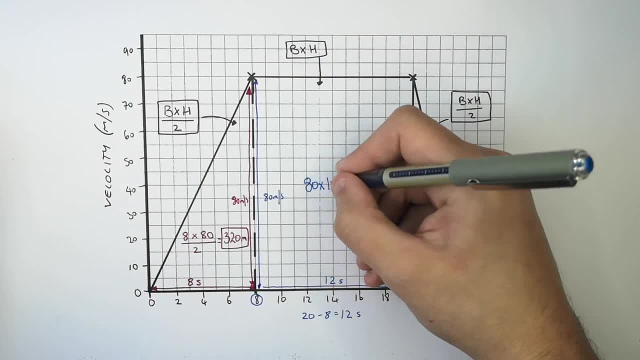 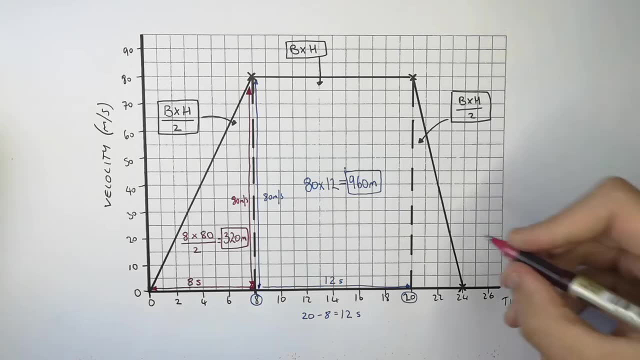 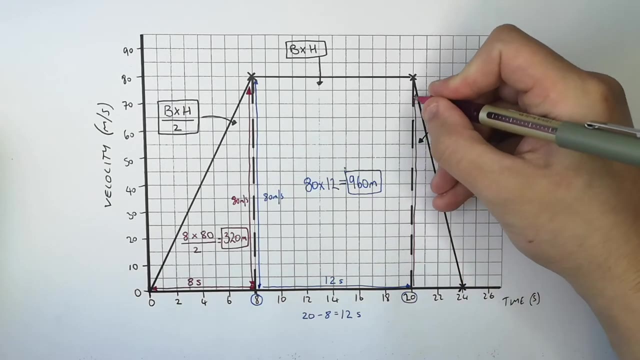 area of the rectangle. you do 80 times 12.. That gives you a distance of 960 meters, And to work out the distance the car traveled while it was decelerating you use base times, height divided by 2.. So the height is going to be 80 meters. 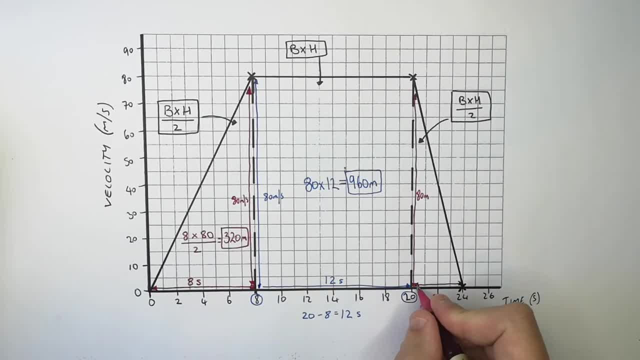 per second. so it's 80. And the base is going to be 24 seconds minus 20 seconds, which gives you a base of 4.. So to calculate the distance the car traveled while it was decelerating, you do 80 times 4 divided by 2.. That will give you. 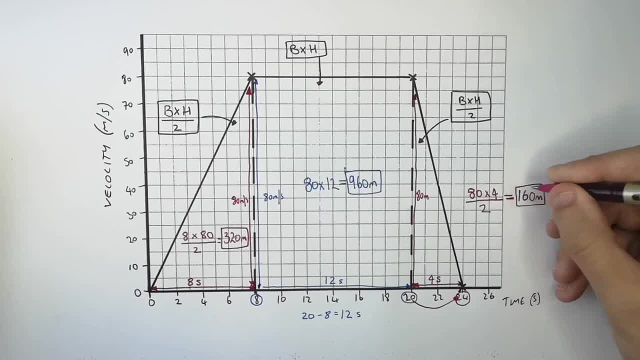 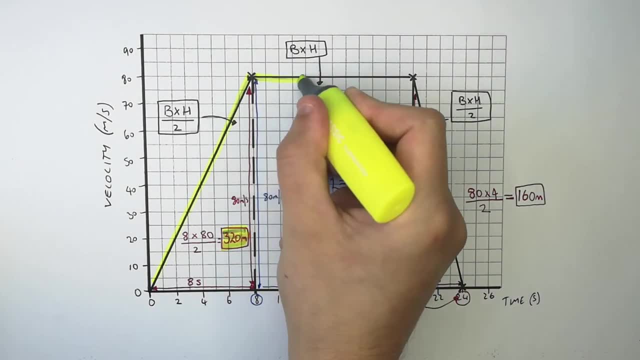 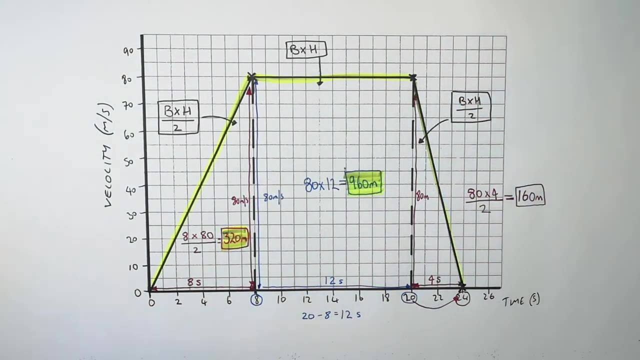 a distance of 160 meters. So while the car was accelerating, it traveled 320 meters. While the car was traveling at a constant velocity, it traveled 960 meters, And while the car was decelerating it traveled 160 meters. So to work out the 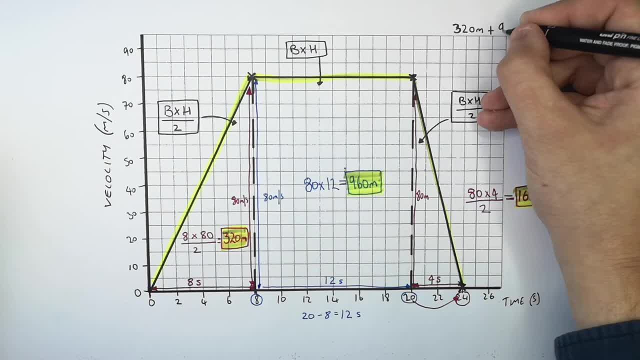 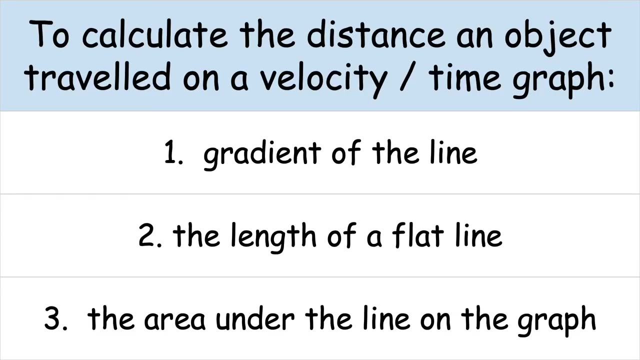 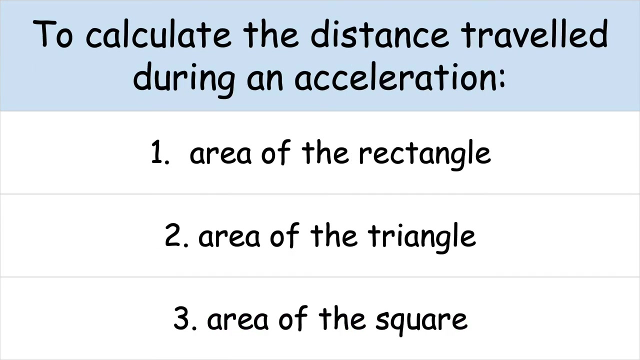 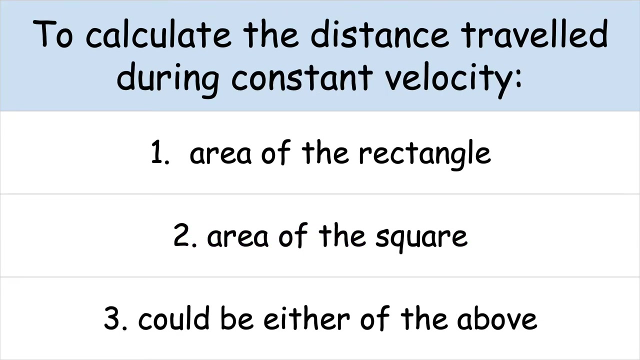 total distance the car traveled, you do 320 meters plus 960 meters plus 160 meters equals 1440 meters. It's question time. Tempt these questions to check your understanding. Let's do that. Step 1. This is the problem you will learn how to solve. Press pause to attempt it. The 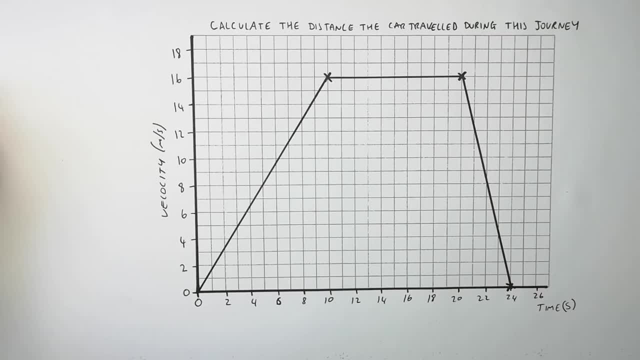 method and the answer will follow. Press pause and calculate the distance the car travelled during this journey. The answers will follow. So to calculate the distance the car travelled while it was accelerating, you use the equation base times, height divided by 2, because it's a triangle that you're trying to work out. the area of 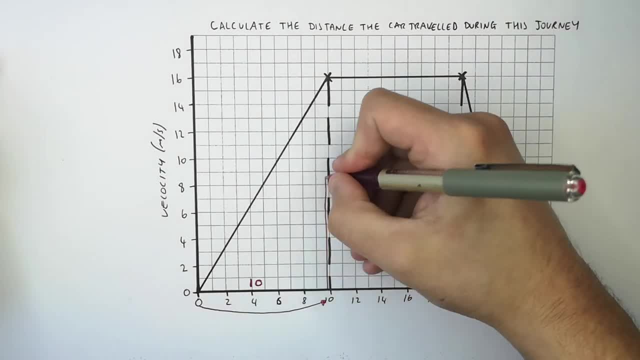 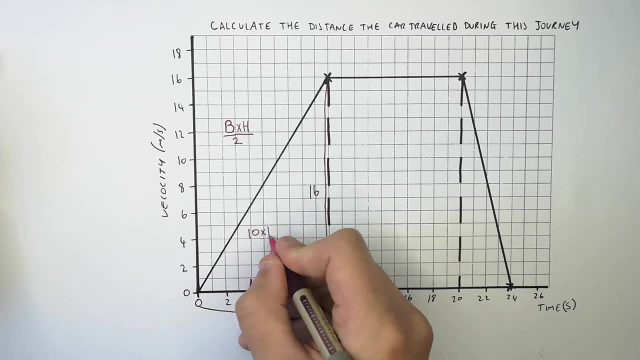 The base is 10, the height is 16.. So now you do base times. height divided by 2, which is going to be 10 times 16 divided by 2, that gives you a total distance during acceleration of 80 meters. So now, because it's a square or a rectangle, you use the equation base times. 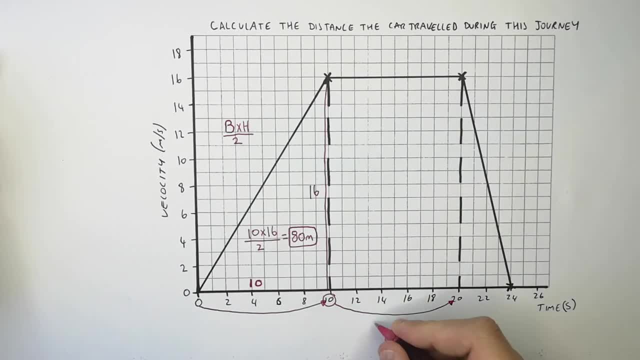 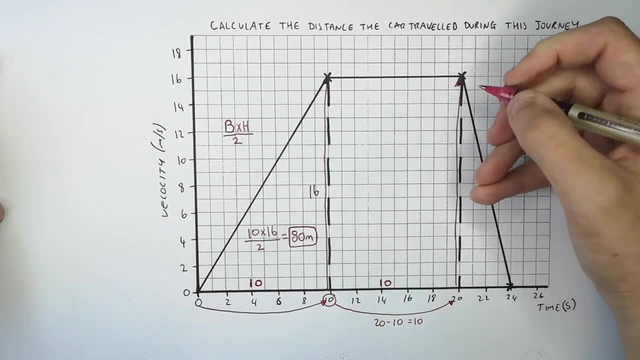 height to work out the area of this rectangle. So the base is going to be 20 minus 10, which is going to give you a base of 10, and you've got a height of 16 meters per second. So that means you use the equation base. 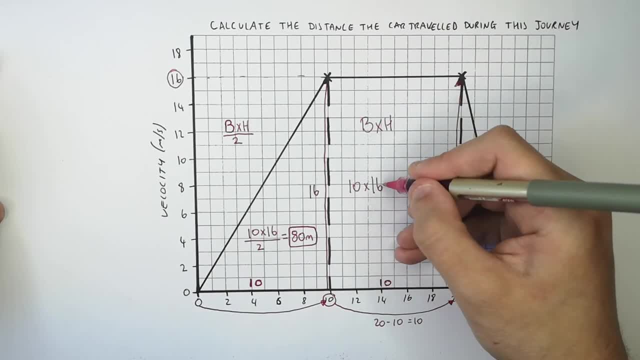 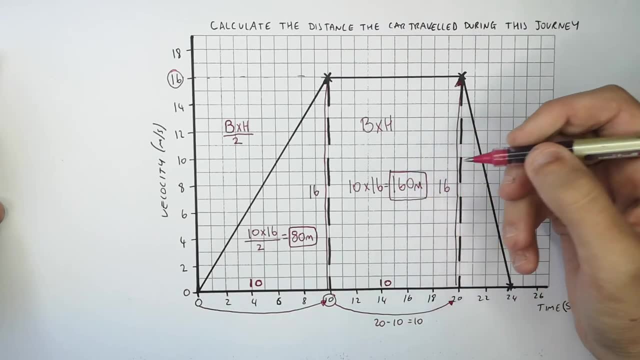 times height, and it's going to be 10 times 16 and it gives you a distance of 160 meters. So the car traveled 100 and 60 meters, while it was traveling at a constant velocity of 16 meters per second. So now we're going to work out the distance. the car 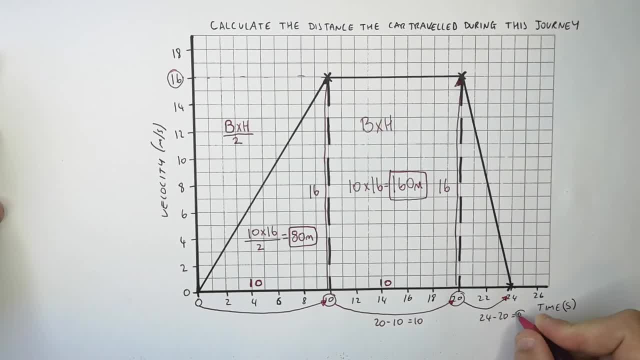 traveled while the car was decelerating. So the base is going to be 4, the height is still 16.. So you do base times height divided by 2, because it's a rectangle. So it's 4 times 16 divided by 2, which. 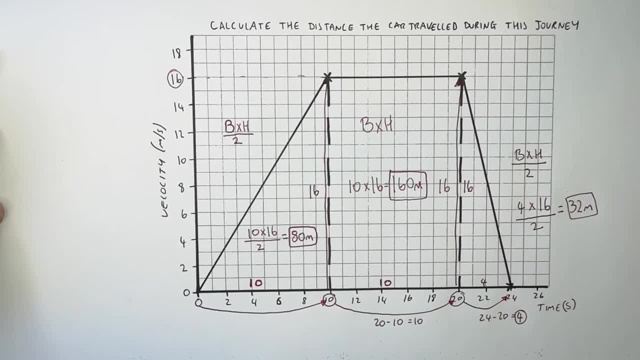 gives you a distance of 32 meters. So to work out the total distance the car traveled, you then do 80 meters plus 160 meters plus 32 meters, which gives you a total distance of 272 meters. That's how far the car traveled during the journey. It's question time. attempt these. 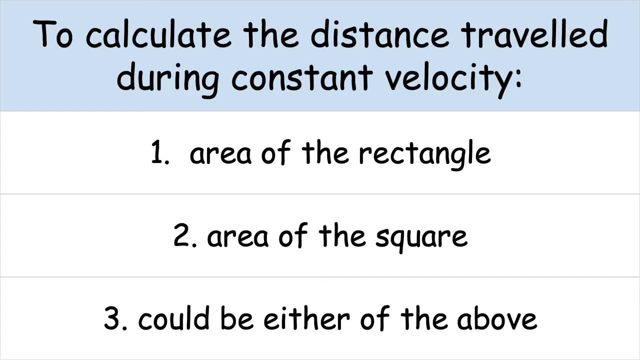 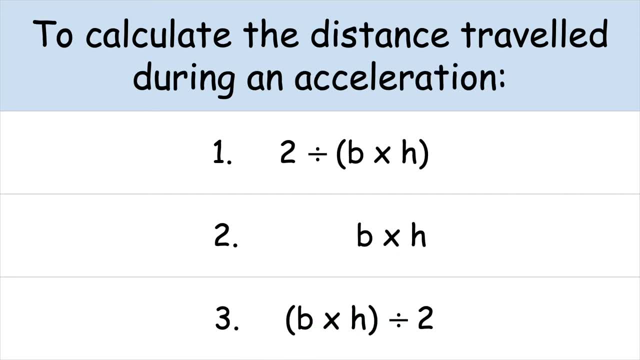 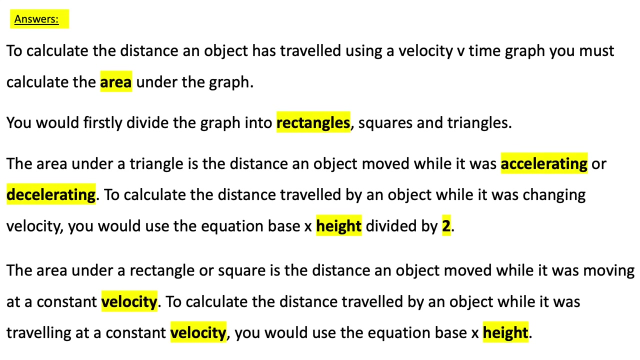 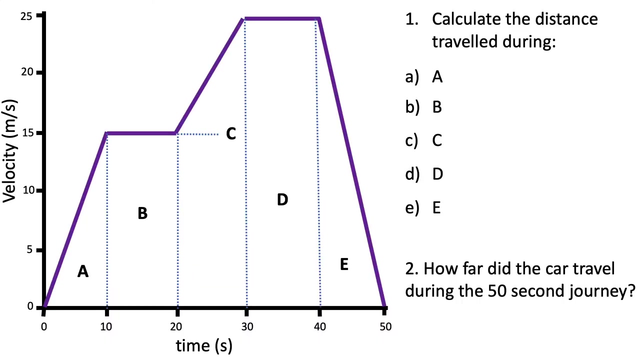 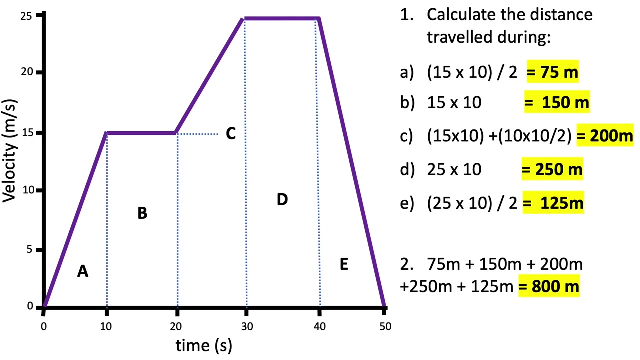 questions to check your understanding. Press pause to let your öğwa pray something. Press pause to let your öğwa pray something and make any corrections to your mistakes. Visit ksciencecom for more free videos, worksheets and quizzes at ksciencecom. 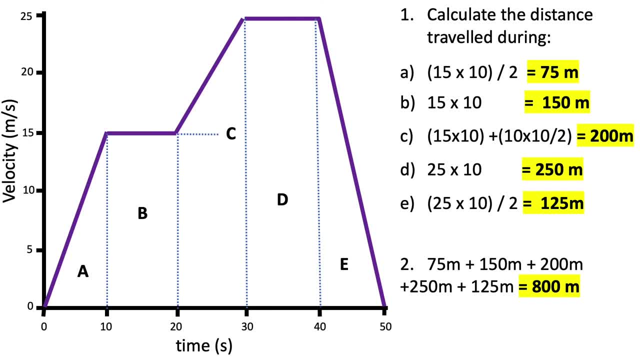 and don't forget to like and subscribe.